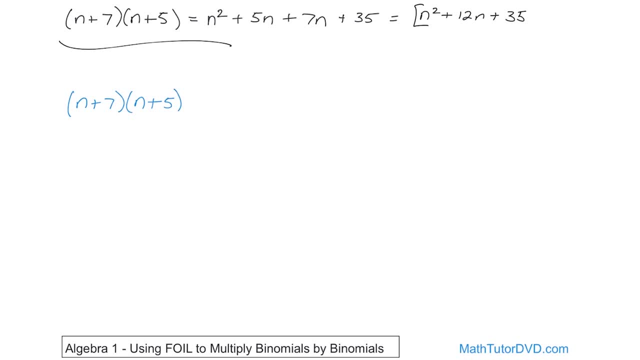 now what I'm going to do is teach you this thing called the FOIL method. So first let's write it down And it's spelled F-O-I-L, And that stands for first, And then it's spelled outside, inside and last. Again, the way to do this. it's not any better or worse than 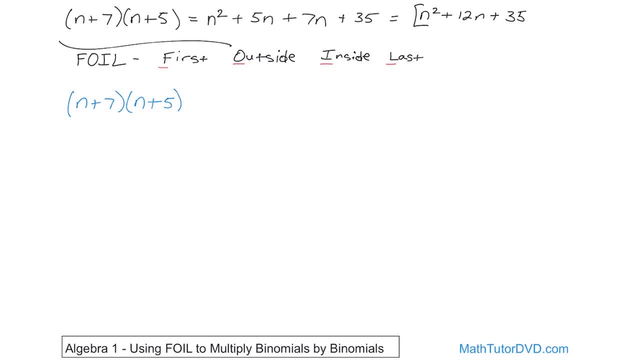 what we've done before. It's just an easier way to remember it for some people. So the way you look at this is: you have a binomial and a binomial. Now what it's telling you to do is you want to multiply the first terms together, Then you want to multiply the outside. 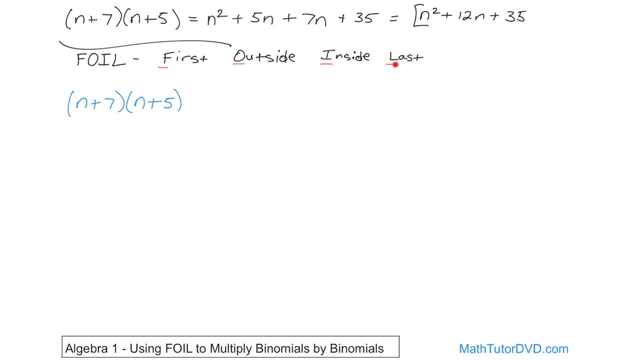 terms together, Then you want to multiply the inside terms together, And then you want to multiply the outside terms together, And then you want to multiply the inside terms, side terms together, then you want to multiply the last terms together. So the first terms are: 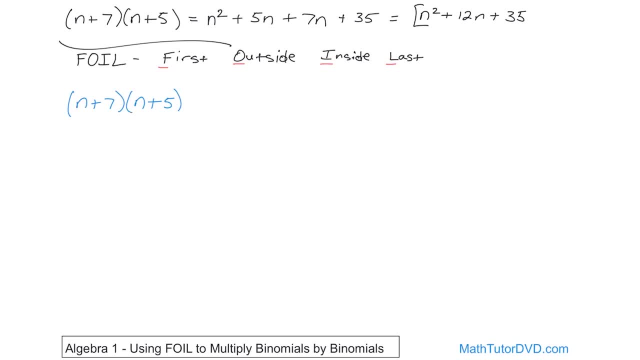 these two. See, this is the first term of this binomial. and this is the first term of this binomial, all right, So if you wanted to draw that, these two terms would be the f terms. Those are the first two terms and you multiply them together, So n times n is n squared, all right? 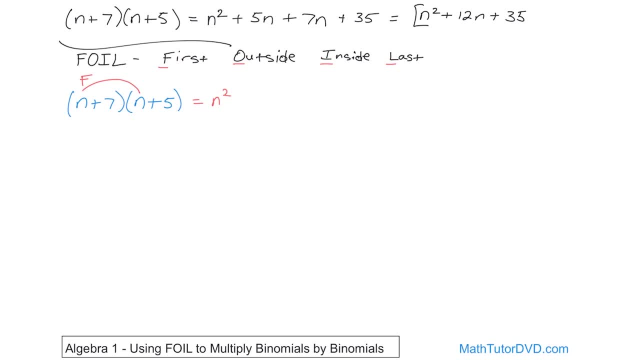 So, when you look at FOIL, it's telling you to first multiply the first terms together, the first term of each binomial, and that's what you get. Then it's telling you to multiply the outside terms. See, these are the inside terms, meaning inside. they're close to each other. If 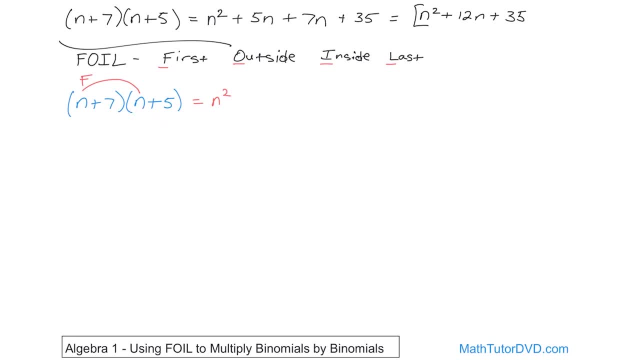 you look at the whole thing, these two are the inside terms and these two are the outside terms. So you would say that these are called the outside terms and you need to multiply those together. So what you have is n times 5 gives you 5n- 5n. okay, Now I'm going to. 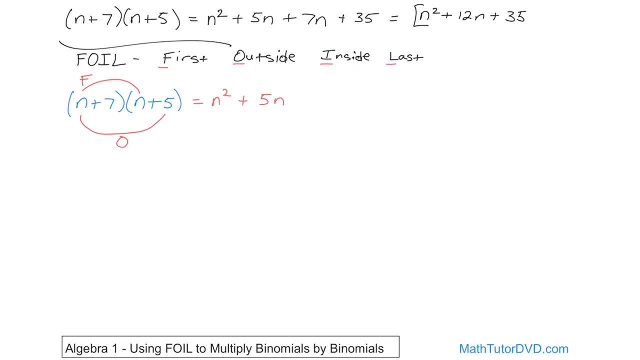 move on to the, the inside terms, which we just talked about. so let's go ahead and mark that down. So here these are called the inside terms. I'll mark that with an i and you multiply those together and you have 7. 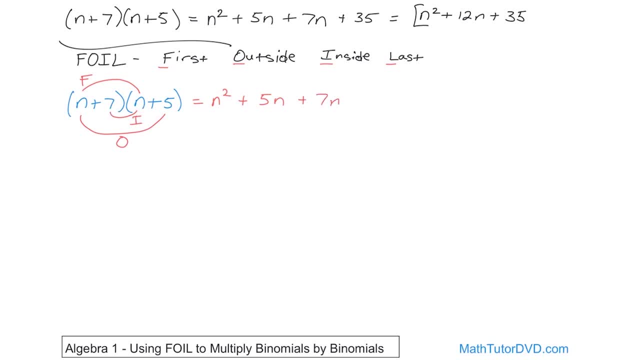 times n, which is 7n, and then you have what we call the last term. So we'll go ahead and draw those together. last, because this is the last term of this binomial. this is the last term here. So 7 times 5 is 35, so you write it down as 35, and I think you can kind of see what's happening. 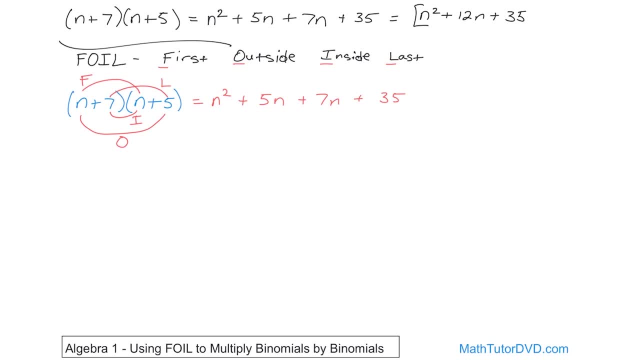 here. When you add these, you get 12,, just like we did before, and so you get n squared plus 12n plus 35.. Okay, and this is the same exact answer. So, whether or not you do it, the 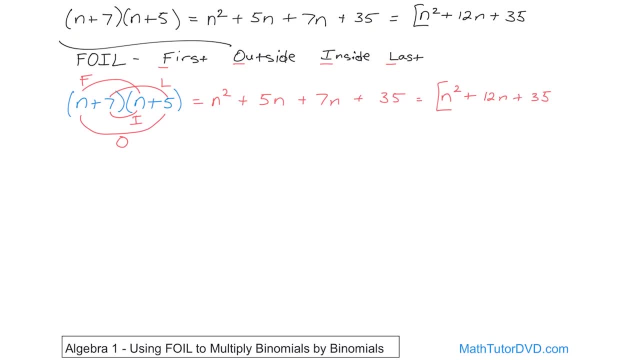 way I taught you in the last section, which is what we did up here as a review, or whether or not you use FOIL. if it's easier for you to remember F-O-I-L, that's okay. You're going to. 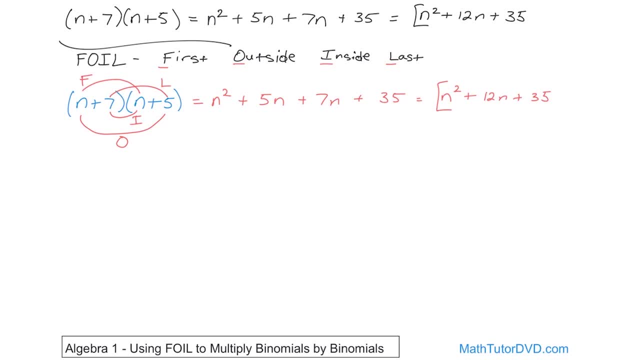 get exactly the same answer, as long as you follow one of these rules, And so your teacher is probably going to teach you this at some point. You're probably going to have to show that you know what FOIL is, but honestly, I don't care which way you use, as long as you get the final answer. 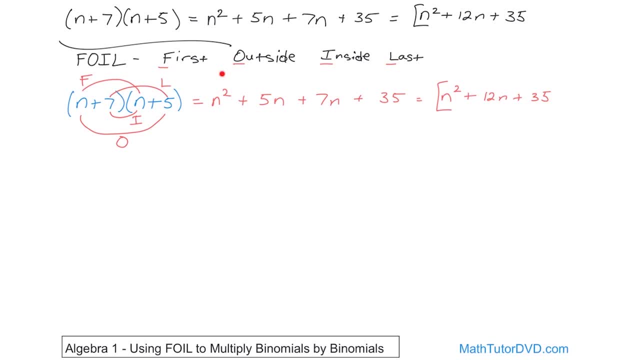 Notice what's happening though. You're getting exactly the same terms. You have n squared here, you have 5n here, you have 7n here and you have 35 right there. So you see, you're doing exactly the same thing in both cases. You're getting exactly the same terms. In fact, I actually 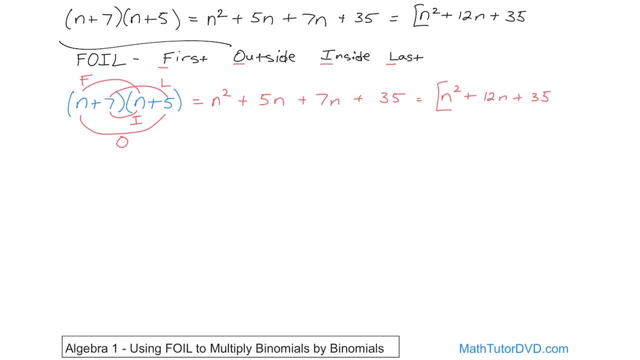 taught you, basically taught you FOIL, without even telling you that's what it is. So here's the first terms. When you distribute this over there, those are the outside terms. Then you go to the 7 and distribute him. those are the inside terms. And then you multiply these. those are the 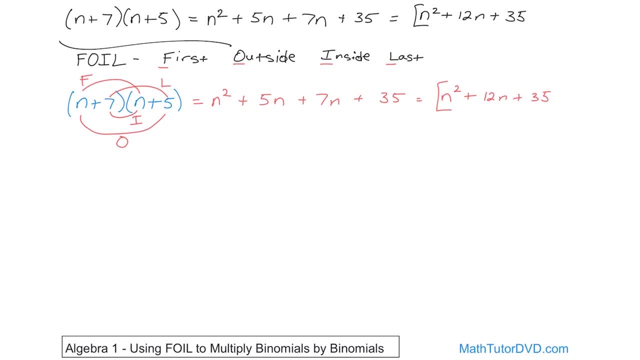 last terms. I kind of taught you that it was FOIL without really telling you that it was FOIL initially. The only reason that I didn't really tell you before is because when people see these words to help them remember, they think it's some kind of shortcut or some kind of trick. And then 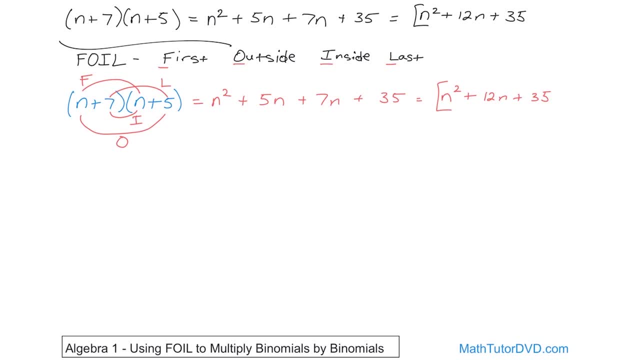 people don't understand the true reason why we're doing it. The reason why we're doing it is because we have two things sitting out here and we're distributing them in, just like we've been using the distribution rule all of this time. So I wanted you to understand that, first and foremost. 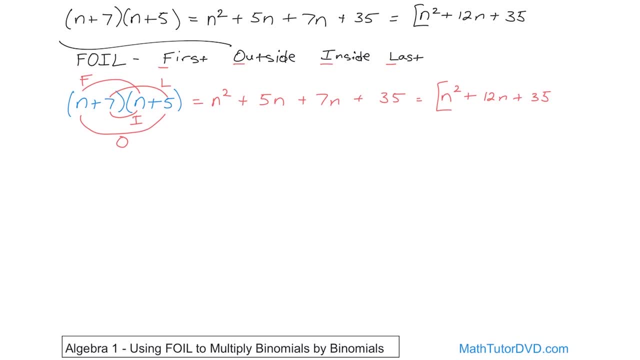 Once you get that, then I can show you: hey, they all have the same terms. You can also call it FOIL, right, All right, so let's just do a couple more problems, get some more practice, and then you'll understand that you're getting the same answer in all cases. All right, 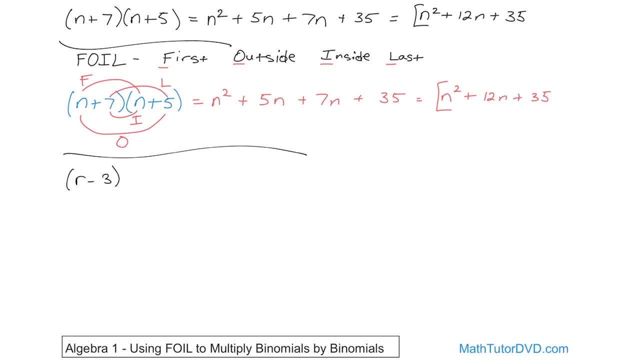 so the next problem is r minus 3, r plus 6.. And we're going to use FOIL this time just to help you remember it. So the first terms r times r is r squared. The outside terms r times 6 is 6r. The. 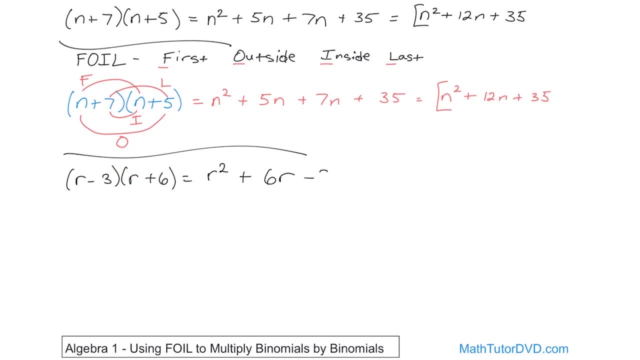 inside terms: negative 3 times r is negative 3r. And the last terms, negative 3 times 6 is negative 18.. Now that we have that done, we combine like terms which are just these: 6 minus 3, it gives 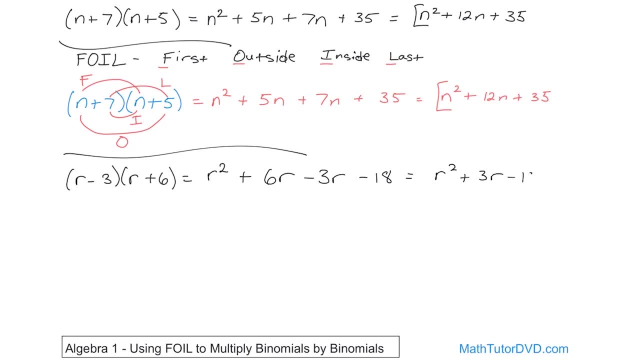 you 3.. So r squared plus 3r minus 18.. Okay, r squared plus 3r minus 18.. Again, you're getting exactly the same thing that we were getting before doing it. exactly the same way, It's just. 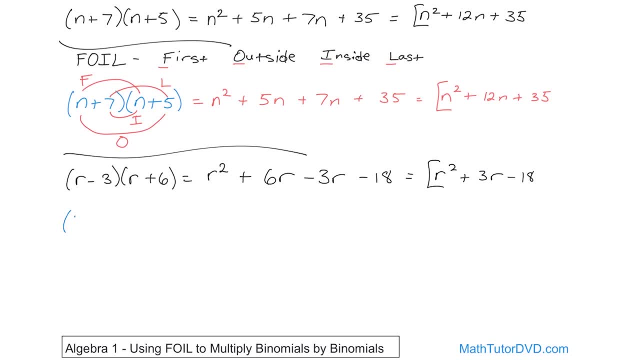 called something a little bit different And it helps some people remember 3a minus 2, a minus 3.. Okay, so we're going to do FOIL right. So the first terms are these two: f. Those are going to be the first two terms. 3a times a gives. 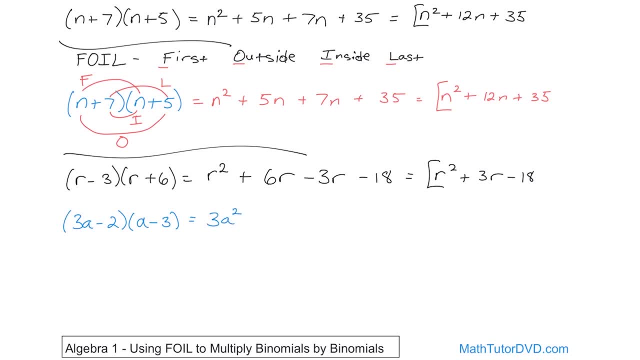 you 3a squared. Then we have the outside terms 3a times negative 3.. Don't forget there's negative 3a times negative. 3 gives you negative 9a. Then we have the inside terms. these two, These are: 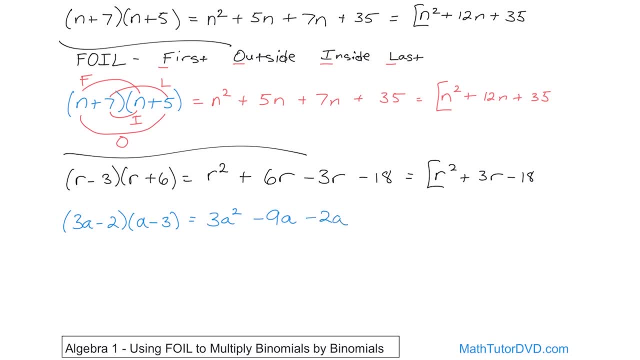 the inside terms: Negative 2a. Then we have the last terms: Negative 2 times negative 3 gives you positive 6. And we combine like terms which are just going to be these two Negative 9 minus 2 is going to give us. 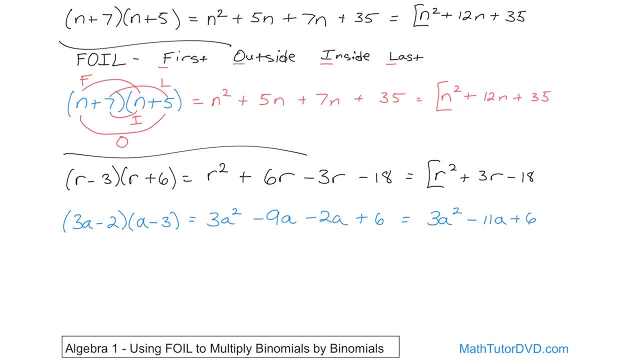 negative 11a like this. So we have 3a squared minus 11a plus 6.. That's the final answer. Now we just have one more of these to get some more practice, And it is 5k plus 2.. 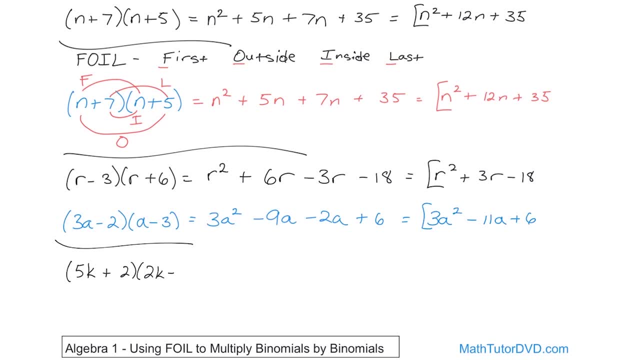 2k minus 3.. All right, 2k minus 3.. And so the first terms, f. these are these terms here. 5k times 2k is 10.. And k times k is k squared. Then we have the outside terms. These are the outside terms. 5k times negative 3 gives you negative 15k. 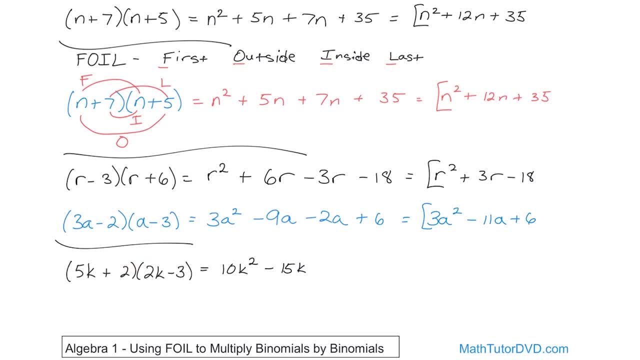 Then the inside terms, Those are the 2 times the 2k gives you 4k, positive 12m plus 5k. And then the last terms: 2 times negative, 3 is negative 6.. And then we combine like terms, which is this one Negative 15 plus 4, so that we add those.